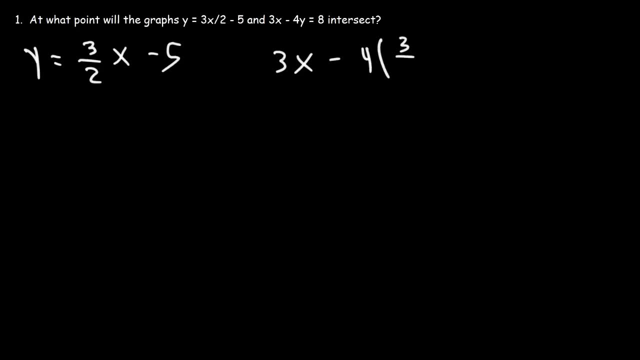 But instead of 4y it's going to be 4 times 3x 3 over 2x minus 5, equal 8.. So let's distribute the 4.. What is negative? 4 times 3 over 2?? 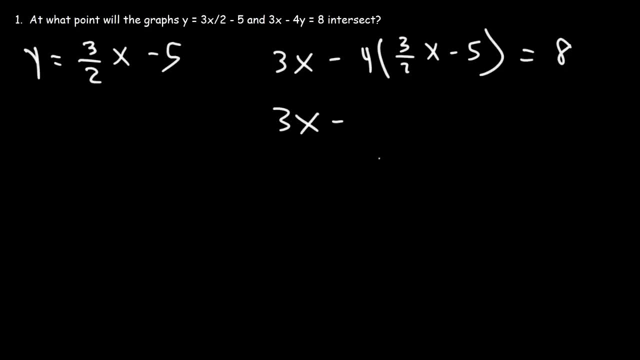 4 times 3 is 12.. 12 divided by 2 is 6.. Now negative 4 times negative: 5, that's positive 20.. So now let's combine like terms: 3x minus 6x is negative 3x. 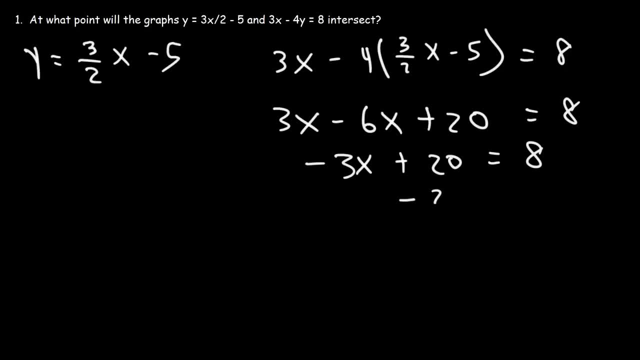 Our next step is to subtract both sides by 20.. So we're going to get: negative 3x is equal to 8 minus 20, which is negative 12.. Now let's divide both sides by negative 3.. Negative 12 divided by negative 3 is positive 4.. 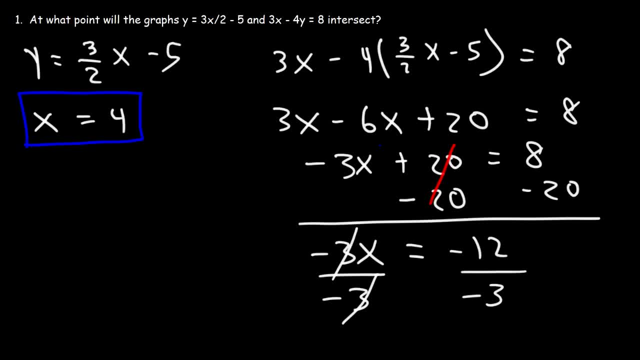 So we have the x coordinate of the point of intersection. Now our next step is to determine the y coordinate. So let's plug in x into that equation. So y is going to be 3 over 2 times 4 minus 5.. 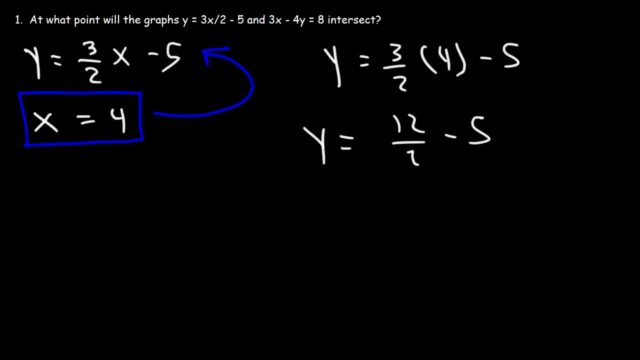 3 times 4 is 12.. 12 divided by 2 is 6.. And 6 minus 5 is 1.. So y is equal to 1.. So we can write the point as So. this, right here, is the point of intersection. 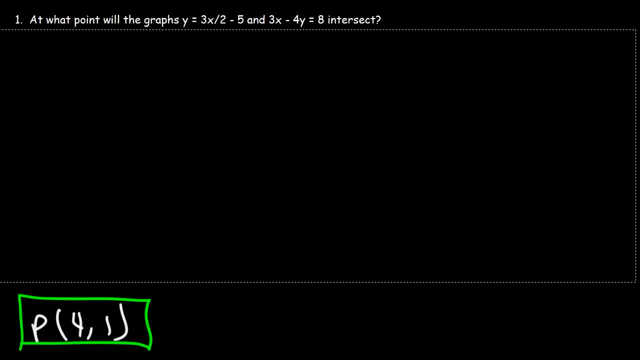 Now what we're going to do is we're going to confirm this answer graphically. Now, before we do so, this equation is in standard form. It's in ax plus by equals c format, And it's better if we convert it to slope-intercept form. 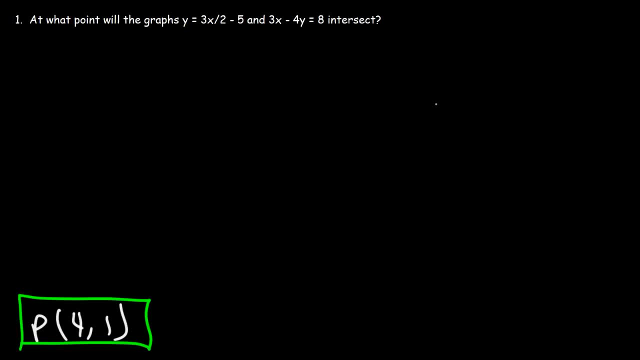 which is in y equals mx plus b format. So let's isolate y in that equation. So first I'm going to rewrite it, I'm going to move the negative 4y from the left side to the right side. On the left side it's negative, but on the right side it's going to be positive. 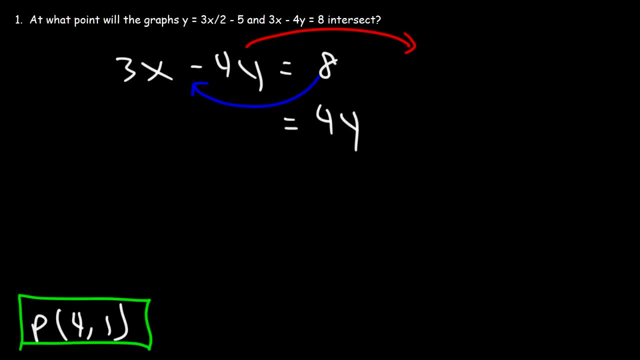 Now I'm going to take the 8 and move it to this side. 8 is positive on the right, but it's going to be negative on the left. Now to get y by itself, I'm going to divide every term by 4..